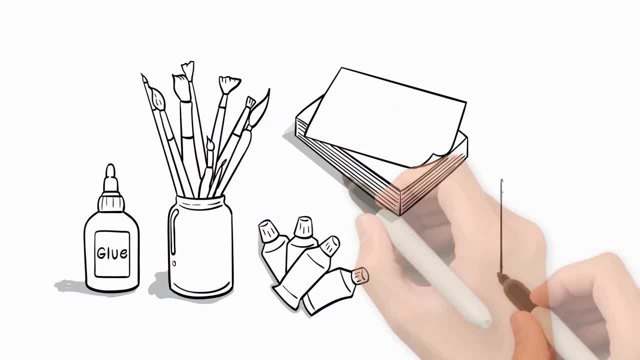 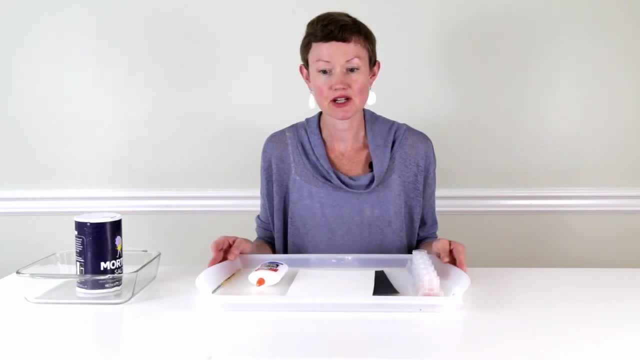 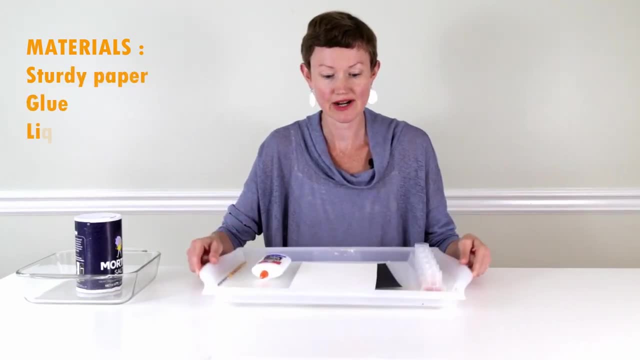 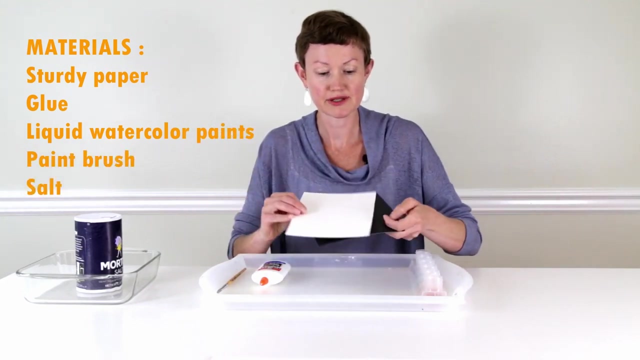 Let's gather our materials. We're going to gather our materials and for raised salt painting, this is what we'll need. We're going to need something to protect the table. I have a tray, some sturdy paper like watercolor paper or poster board, a bottle of glue, some liquid watercolor paints. 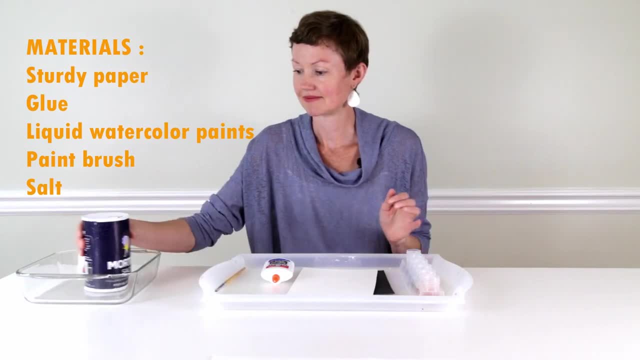 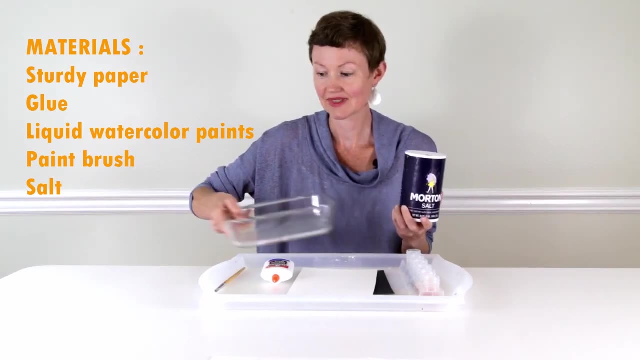 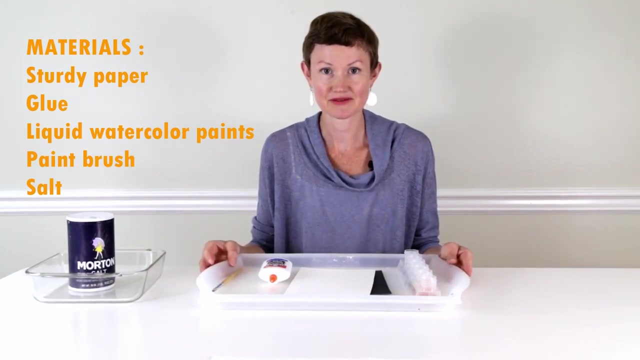 a paintbrush, lots of salt and a baking dish to put the salt in. So not that much. but why don't you go gather your materials now so we can do this art activity together? It's time to set up for success. 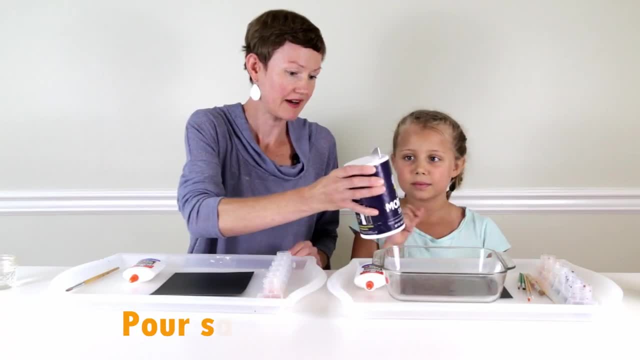 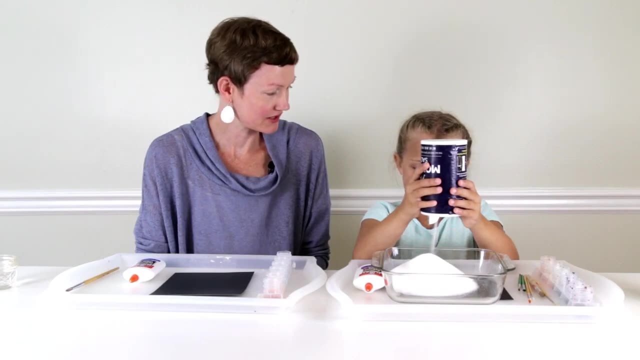 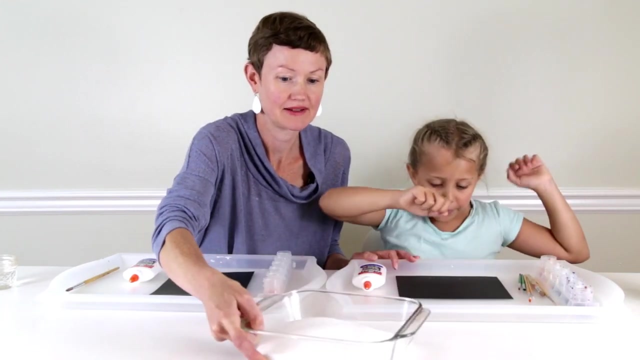 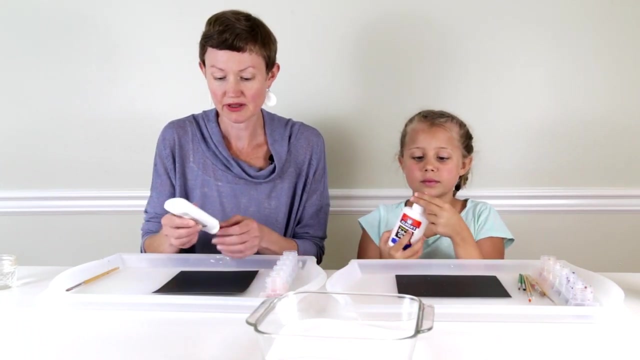 We're going to pour our salt into the baking dish. Daphne, would you like to do that? Mm-hmm, And you can pour all of it in. We'll do a lot of raised salt painting, Okay. So now we're going to set our salt aside. We don't need it quite yet, and the first thing we're going to do is draw a picture on our paper with our bottle of glue, and we use white Elmer's glue or school glue. 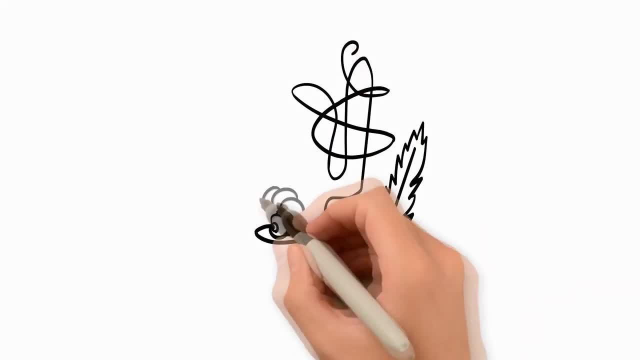 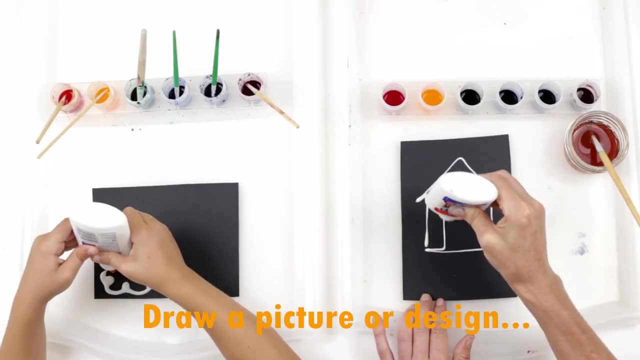 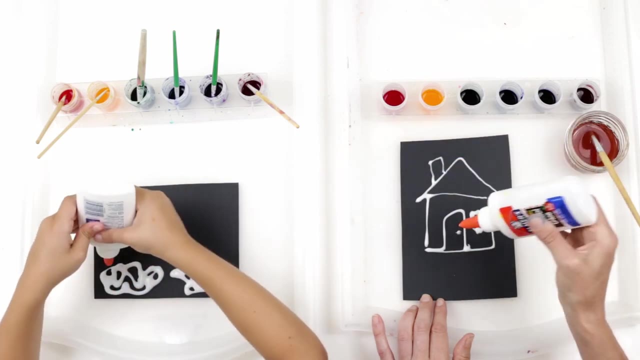 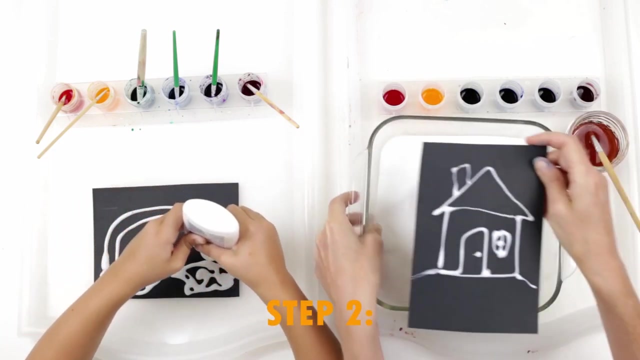 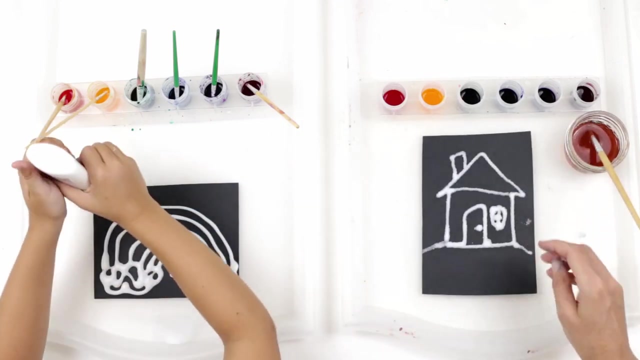 Let's create To make our raised salt painting. we're going to start by drawing a design with the glue bottle onto card stock or heavy paper and then sprinkling salt over that glue design and shaking the excess salt off until your glue design is covered with salt. 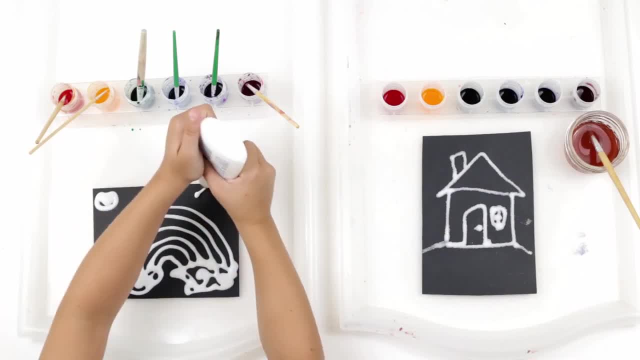 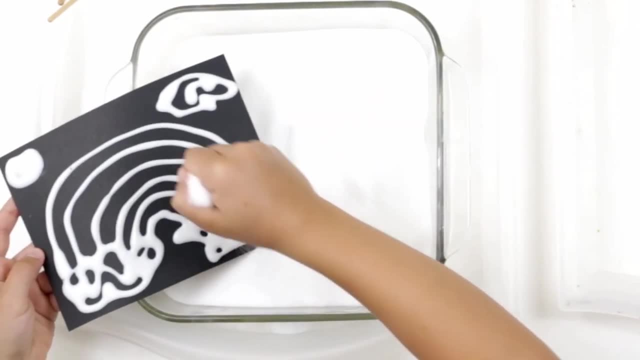 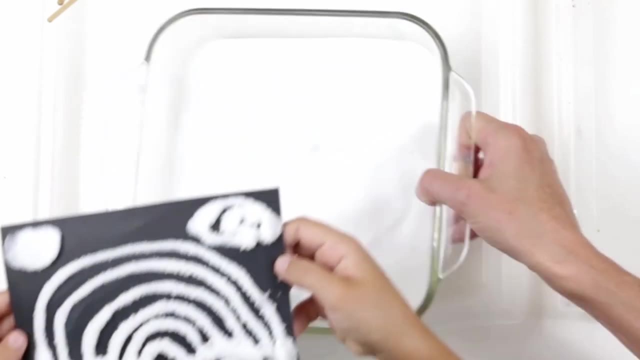 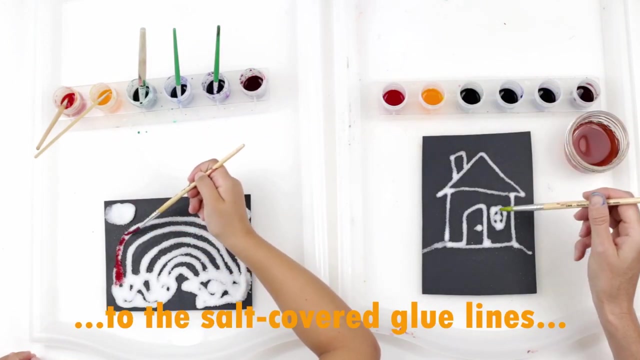 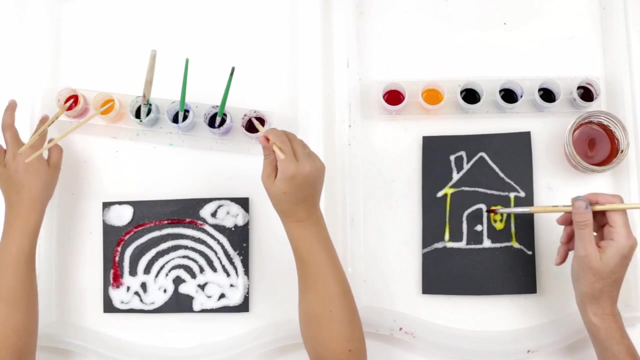 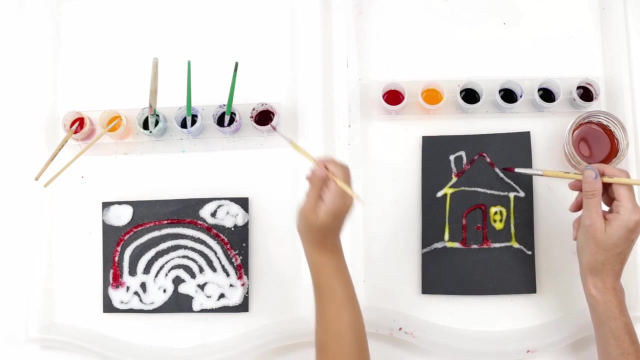 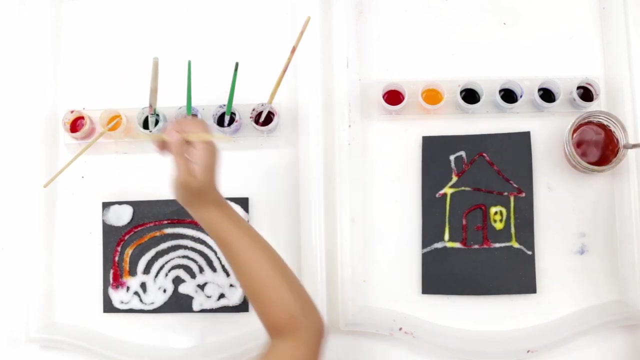 Okay, and then you will take your paintbrush and dip it in the liquid watercolor paint and then touch, gently touch the paint soaked paintbrush to one of the salt covered glue lines and watch as the paint travels along that salt covered glue line. and this happens because of the wicking action of the salt. 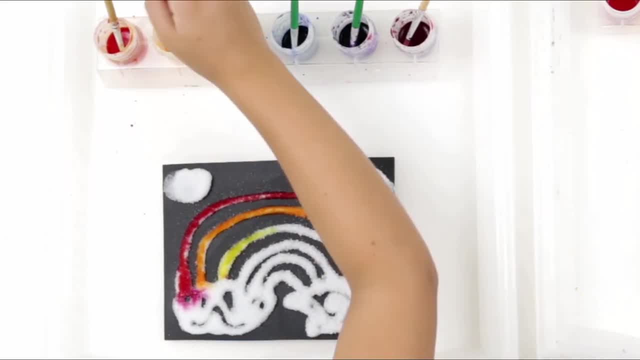 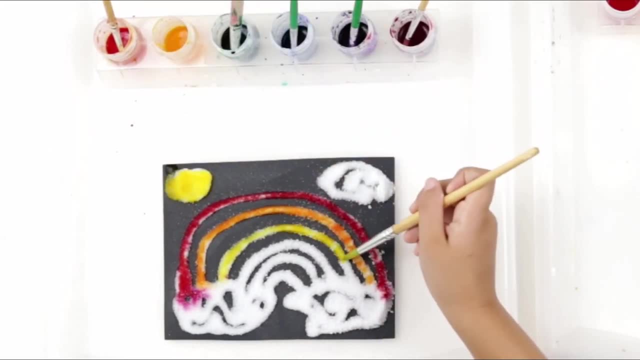 so continue with the different colors of watercolor paint, as many colors as you like. you can do this with just a couple colors, if you like, or the whole rainbow of colors, and continue until you are happy with the design and then set it aside to dry it. 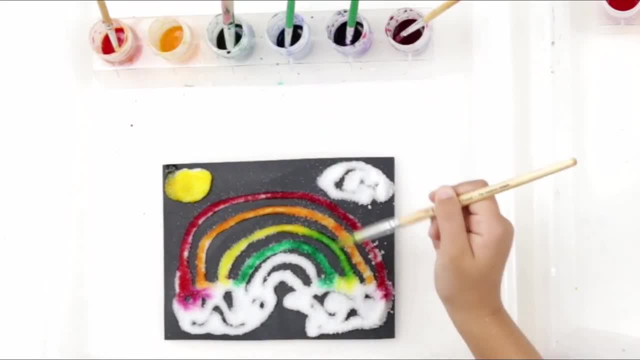 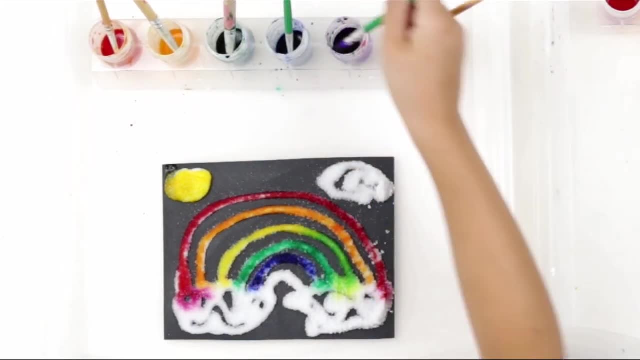 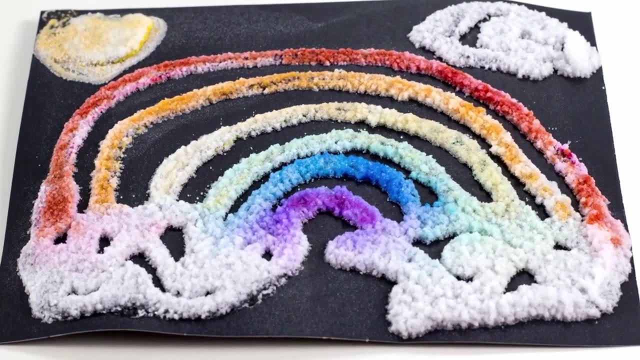 will dry. it will take overnight at least to dry, depending on how much glue was used and how much paint, and then you can, after you set that one aside, you can start a new one if you like, make as many as you like, and once these dry, they dry hard and crystalline. 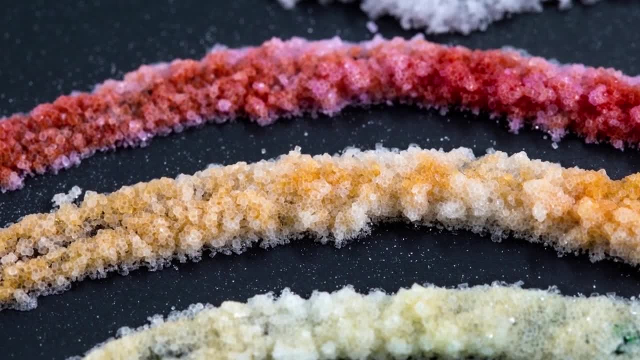 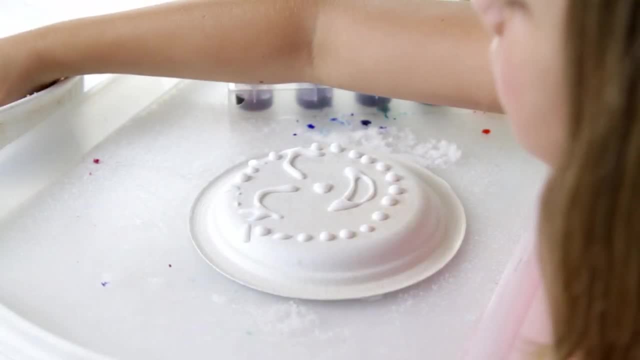 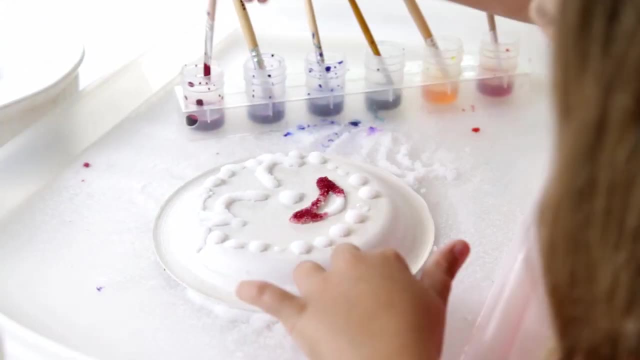 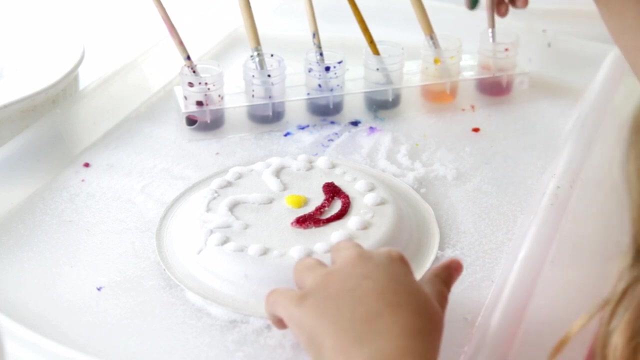 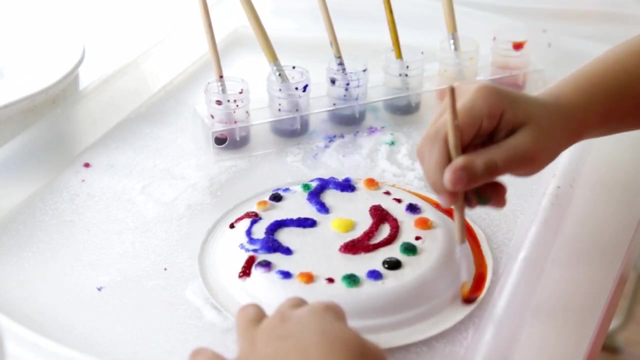 beautiful, sparkly paintings of glue and salt and watercolors, and you can do this with abstract designs, squiggles, scribbles. you can do it with faces, pictures, anything you like. I've been a little lucky and I hope you enjoy this video, guys, thanks for watching.